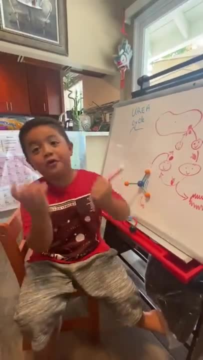 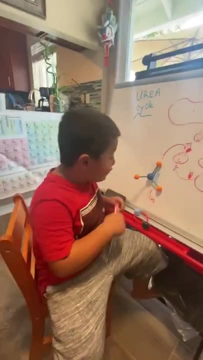 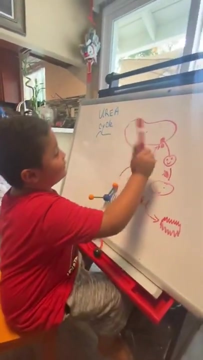 Hi kids, it's Alex again. Today we're doing the urea cycle. kids, You wonder what is a urea cycle That gets rid of the nitrogenous waste? All that money, huh, kids. So we need the mitochondria. 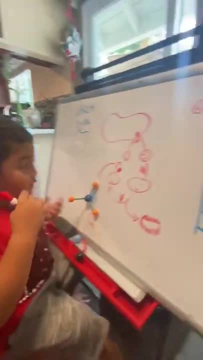 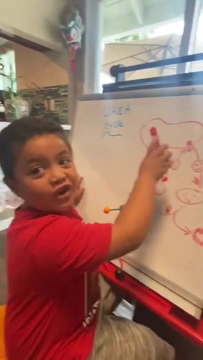 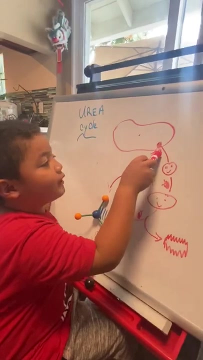 So what are we waiting for? Let's start. Ornithine plus carbamoyl phosphate- Right, That's what the mitochondria is for. Carbamoyl phosphate it's inside of the mitochondria, But make sexually how Ornithine transcarbamoylase- See that word a lot. 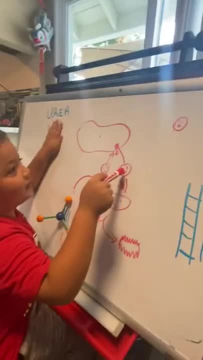 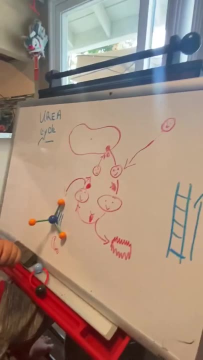 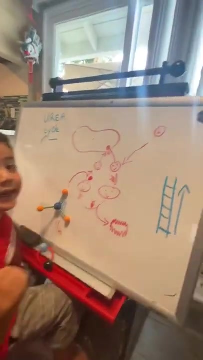 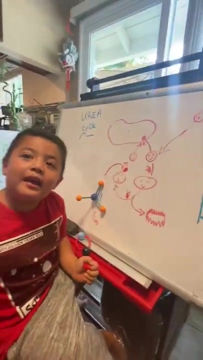 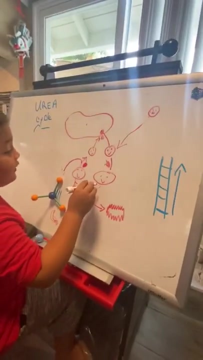 No Ornithine, here comes aspartate to join with sexually kids. To make what? Argininosuccinate? How? Argininosuccinate, Synthetase- kids Say that word a lot. No Argininosuccinate, And now, kids, argininosuccinate is going to become arginine. How? 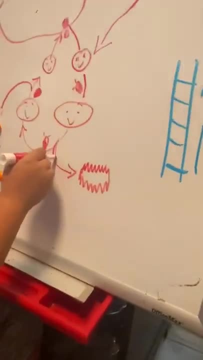 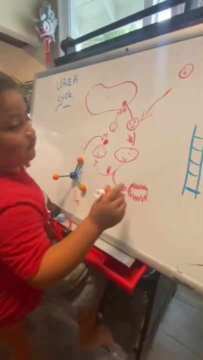 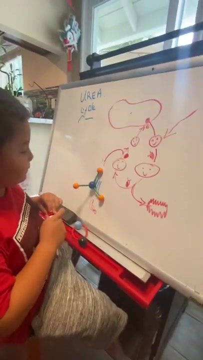 Argininosuccinate, kids And who comes out Bure? It's a Krebs cycle, kids. Check my Krebs cycle video. And fumarates are going to blow up the gluconeogenesis pathway. kids. Now the final steps. 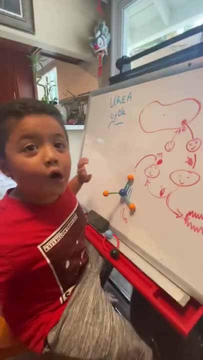 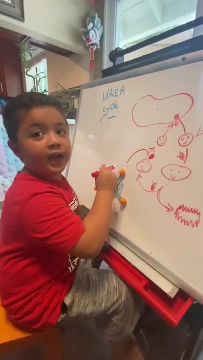 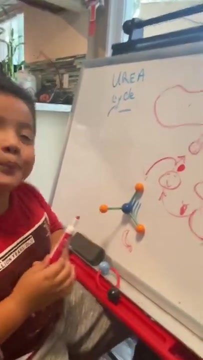 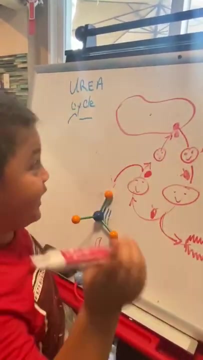 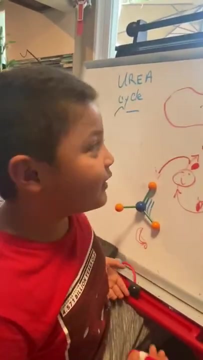 Now arginine is going to go back to ornithine- How Arginase kids. And urea comes out and gets rid of the nitrogenous waste. But let's say One last time: Ornithine plus carbamoyl phosphate makes citrulline. How Ornithine transcarbamoylase kids. 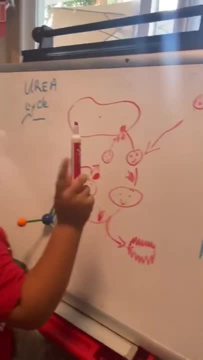 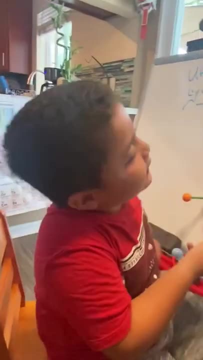 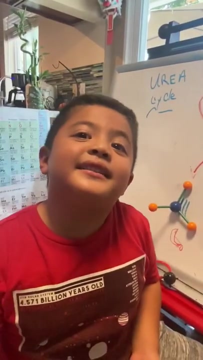 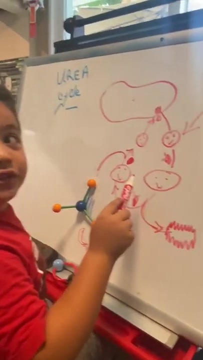 Now here comes aspartate to join with citrulline to make what Argininosuccinate kids. Check my Krebs cycle video. Nitrogenous exp- Chat kids. Arginine is a secondary ingredient And this is a fun fact.